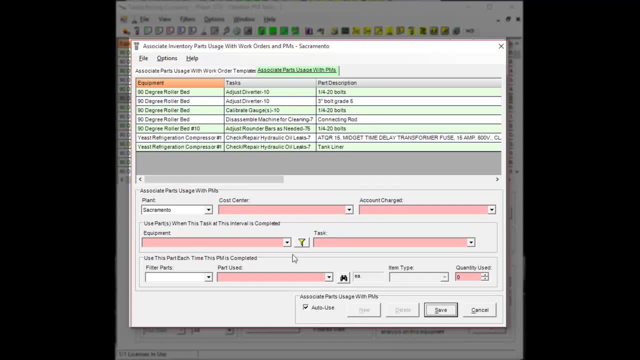 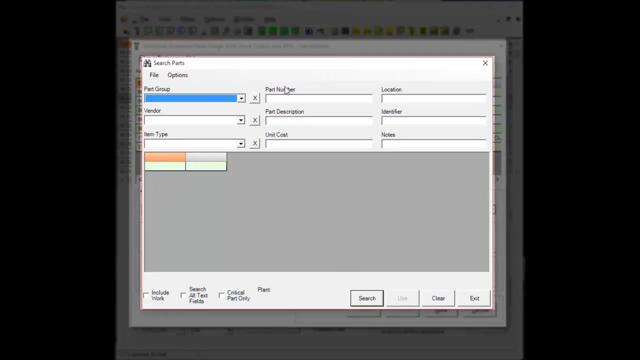 and the task. I'll just pick any to show you as an example. So pick your equipment, Pick the task, Pick the part that you're going to be using by using the search feature. here You can key in everything as necessary And then press search and pick what you need. 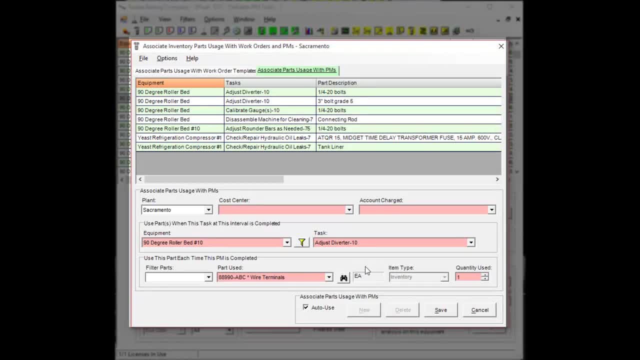 And select the quantity that you'll be using. If you haven't set up your defaults on this page, you'll also have to select your cost center and your accounts. Once all the required information has been filled in, press save And it'll get saved. We're going to close out of this now. 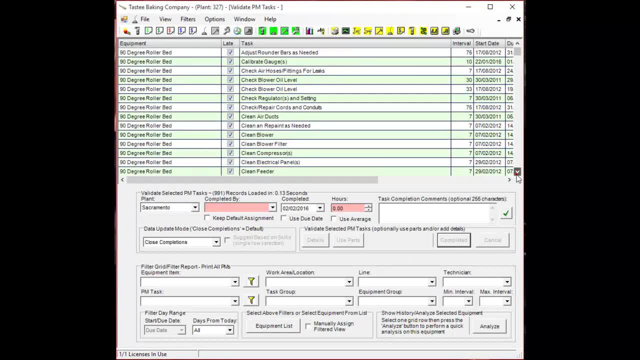 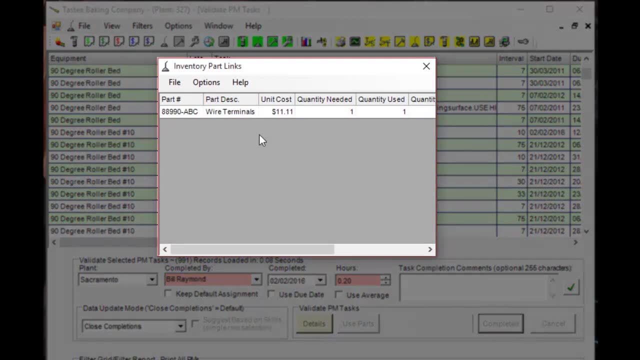 Now we're going to find that PEM task that we just associated a part to right here And we're going to complete it. A new window will show up. This notifies you that a part was automatically used upon completion of this PEM. It shows you that this is the part that was used. how many was used? 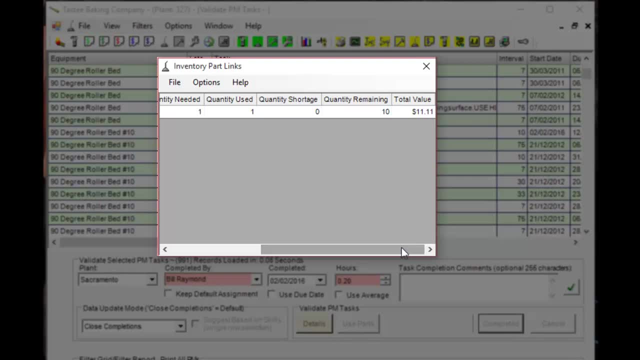 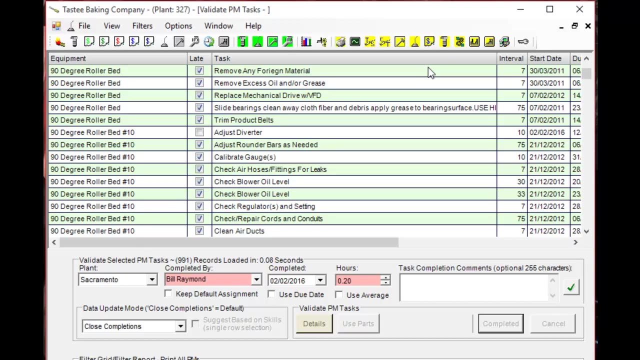 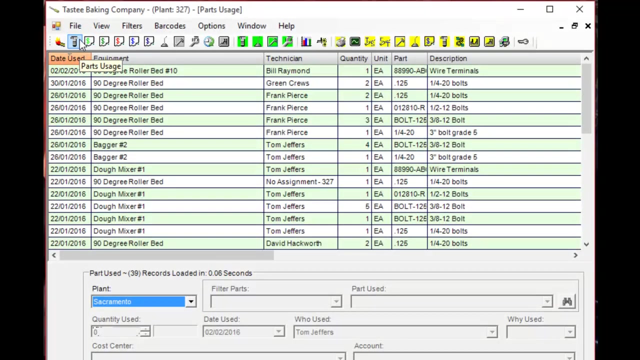 and what the quantity is remaining in stock. If we go to the parts used screen, you'll see that an entry was automatically generated by Mainsmart to use this part. Take a look at the very top And this is the same part that we used for that PEM. 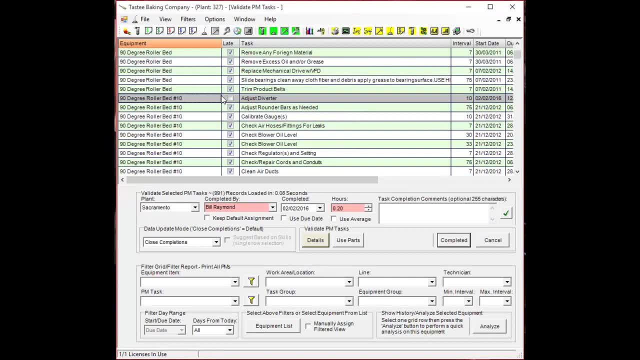 If you're going to be printing this task and emailing it to someone or giving it to a technician and you want them to be able to see the part that they're going to be using when they do this task, select your task, right-click and press print selected PEMs. 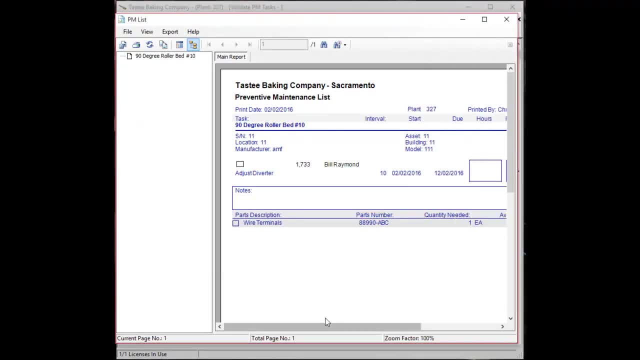 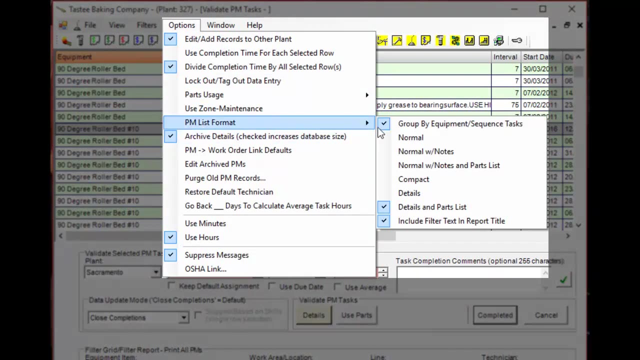 And, depending on your report format, the part may or may not show up. In this case mine did, But I'll show you where you can find that. You can go to options. You can go to the PEM list format And you can pick the one that you need.